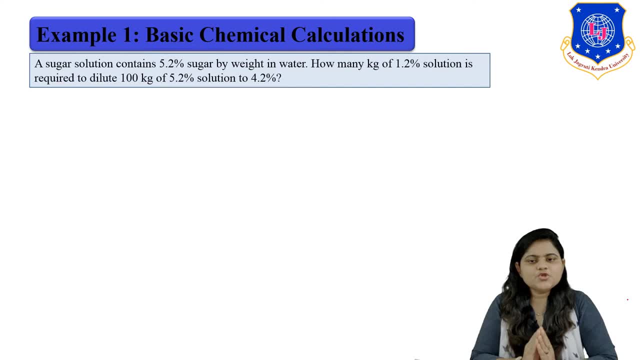 Red Kilogram of 5.2% solution to 4.2%. right Now, see first explain what we need to find out Right? So a sugar solution which contains 5.2% sugar by weight in water. So case number: 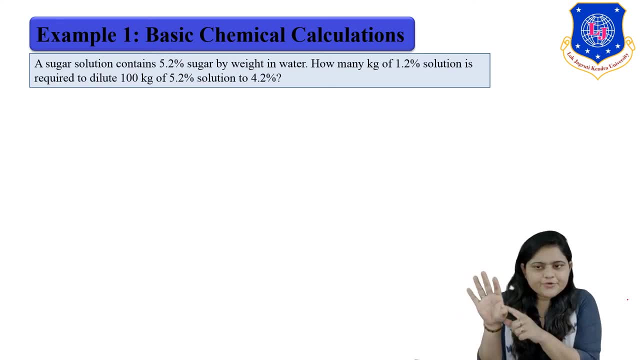 1. a solution is given. In that solution, 5.2% sugar is present Right Now. see what process we have to find out. so we have Here a sugar solution is made in water. so one thing is very clear: our solution consists of. 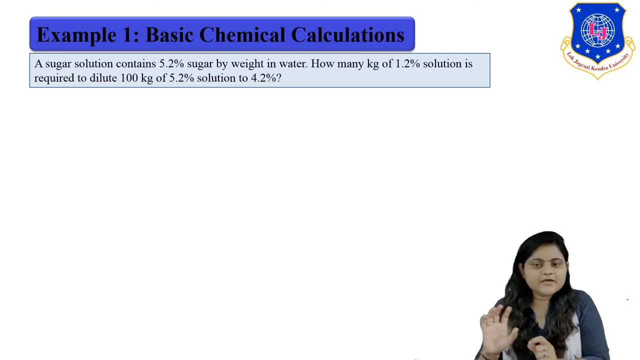 sugar and water. So in case number one, or I can say in a weaker number one, a 5.2 percent concentration sugar is there. remaining will be our water. Now we need to dilute that 5.2 percent sugar to our 0.2 percent sugar. so for that we are adding 1.2 percent solution, right? So how see? 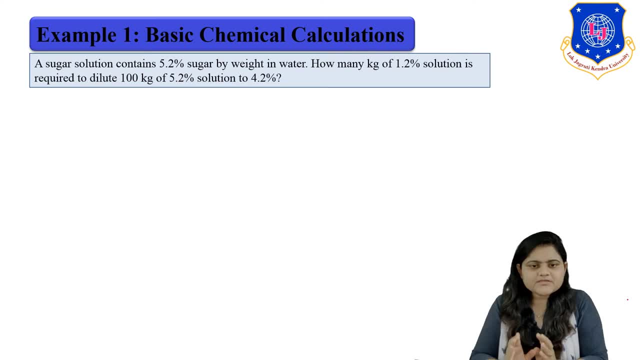 how many kilogram of 1.2 percent solution is required to dilute 100 kilogram of 5.2 percent solution. So here one thing is also: given that the 5.2 percent sugar solution amount is 100 kilogram, right? So simplify meaning of this is like that: a 100 kilogram of 5.2 percent sugar 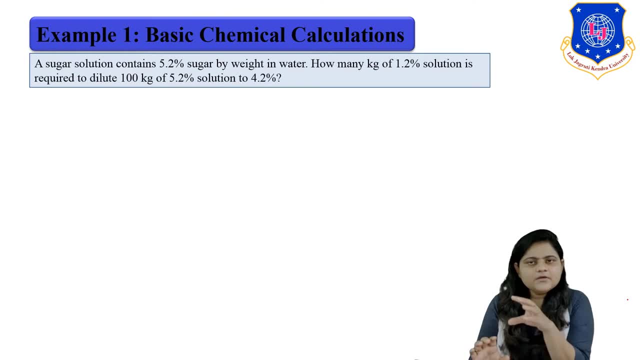 solution is with us. Now we need to add some unknown quantity of 1.2 percent sugar solution to make them as 4.2 percent sugar solution. So we need to find out that unknown quantity of 1.2 percent sugar solution. So weaker number one say: 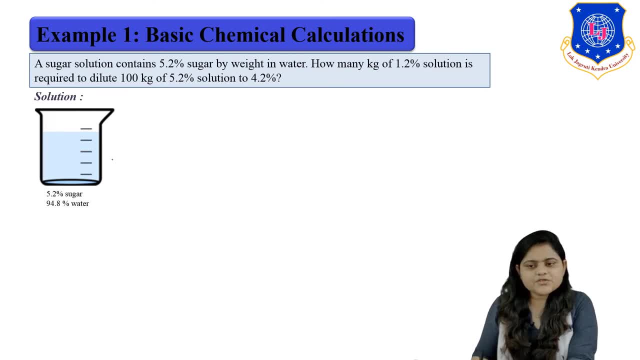 for example, in this weaker a 5.2 percent sugar solution is there, so remaining will be, but of 100 kilogram. Now in this solution of 1.2 percent sugar solution is added to make them as 4.2 percent. Now in this i am adding a 1.2 percent sugar solution, so but 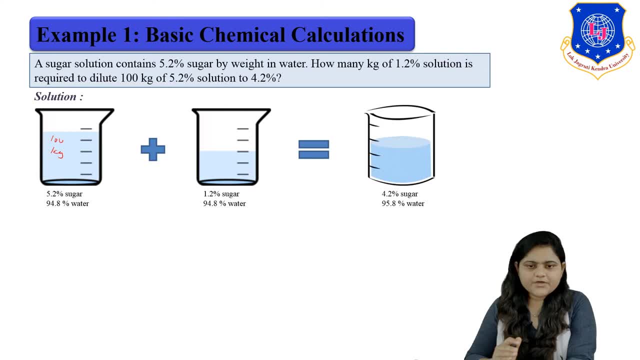 obvious. rest of the amount will be of the water to make them as 4.2 percent sugar solution. Here 1.2 percent is the amount of the sugar, so remaining 98.8 percent will be of water to make them as 4.2 percent sugar. so remaining will be 95.8 percent. 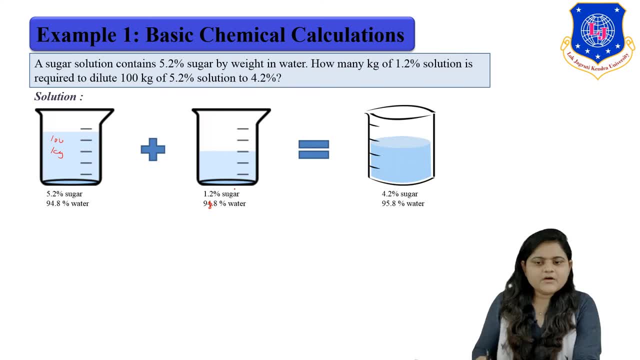 of the water. now what we need to find out. the amount of this solution is to be required, right? so let us assume this is given as 100 kilogram. assume this one is x kilogram and final output is a y kilogram. briefly, i'll give you a pathway how we'll solve this numerical c. 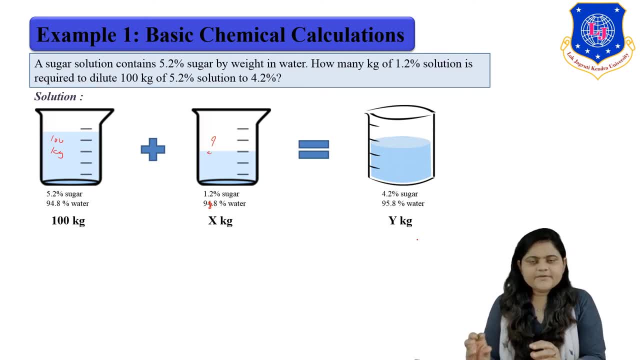 our 100 kilogram is a initial beaker. now in this 100 kilogram we are adding x kilogram of 1.2 solution. so this combinedly will make y kilogram of 4.2 percent solution. so one overall material balance equation i can see here is: 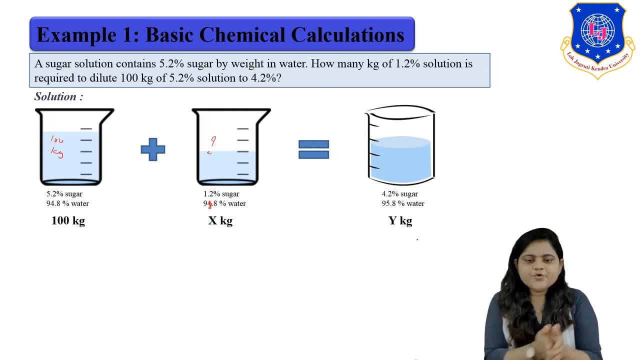 100 plus x will give me y right. so this will be my equation number one. now equation number two. so what will be? i can give equation number two amount of sugar in beaker number one plus amount of sugar in beaker number two, which is equal to amount of sugar in beaker number. 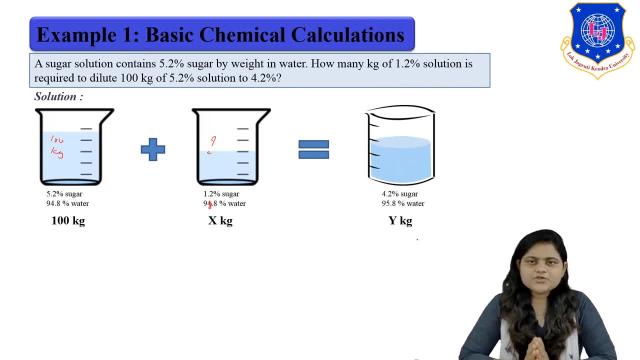 three or i can say final solution. so we have to know exactly such a solution. if we know x and y, then we can find out the value of xfle and yjal. so, my Dr mothers, you mean x kilogram of 1.2 percent solution is required and y aquarium of 4.2. 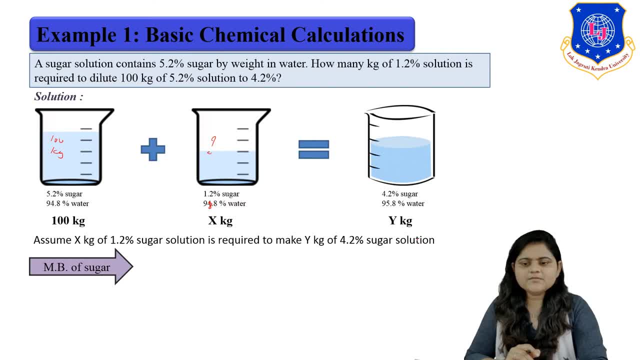 percent. solution is what? so now we will do first material balance of sugar. here i mean material balance of sugar. that means kilogram of sugar, or what number I have distributed around input and exit of mineral sugar in beaker number 1, plus kilogram of sugar in beaker number 2, which is equal to. 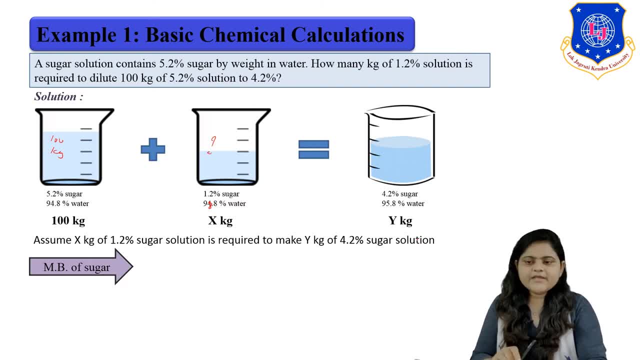 kilogram of sugar in beaker number 3. So in first beaker a sugar present is 5.2 percent, right, but entire quantity of our solution in first beaker is 100 kilogram. So in that 5.2 kg is sugar in first beaker and 94.8 kilogram is water. So sugar in this plus. 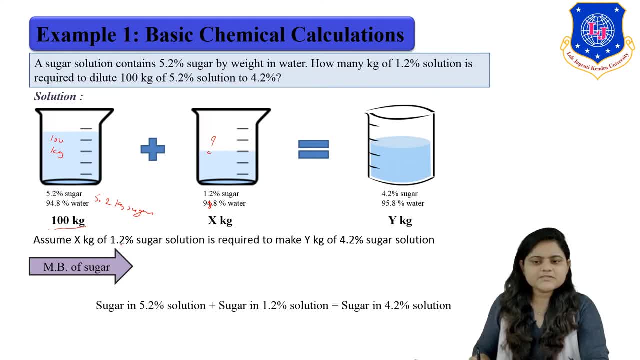 sugar in 1.2 is equal to sugar in 4.2 percent solution. So sugar in this will be 5.2 kilogram plus amount of sugar in beaker. number 2 will be 1.2 percent of x right, So 1.2 percent. 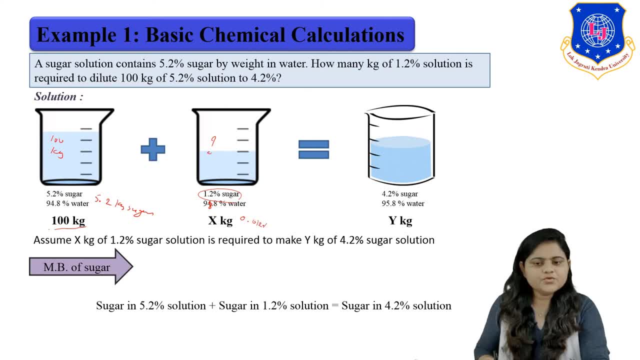 of x will become 0.012 x, and here the amount of sugar in final solution will become 0.0425, right? so it will become like this: 0.052 multiplied by 100, which is nothing but the 5.2 plus 0.012 x is. 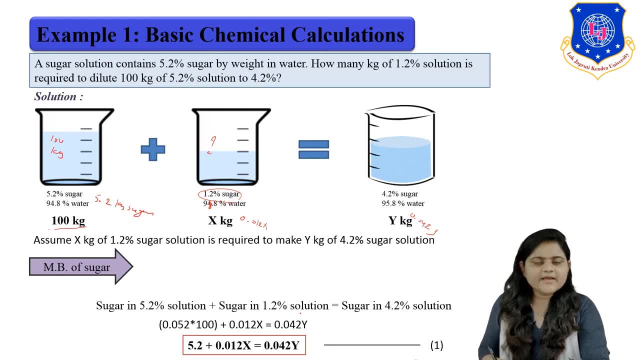 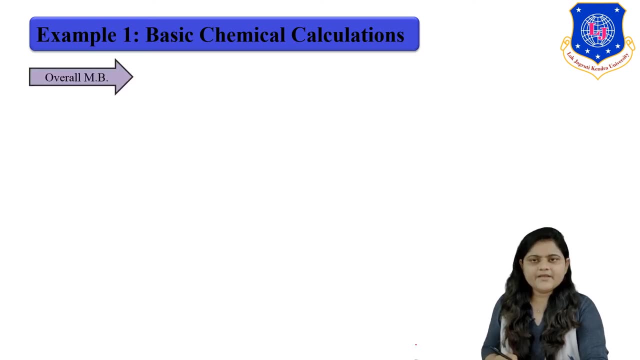 equal to 0.0425. simplify these and give this equation number 1. now we have two unknowns, so we need to find out one more equation. that equation i can clearly see here: overall material balance. overall material balance, that means 100 plus x is equal to y. see, now we have two. 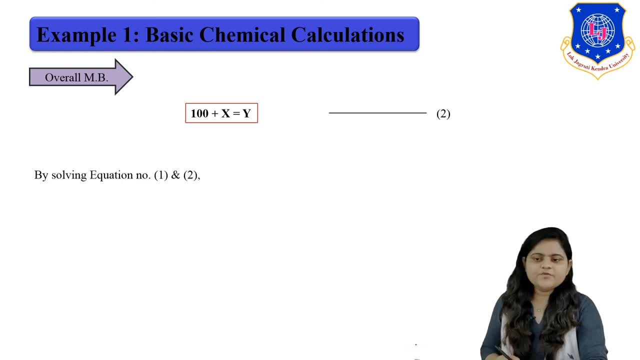 equations: equation number 1 and equation number 2. by solving this two equation- equation number 1 and 2- we will get. x is equal to 33.33 kilogram. here we need to find out how many kilogram of 1.2 percent sugar solution is required. here we are. 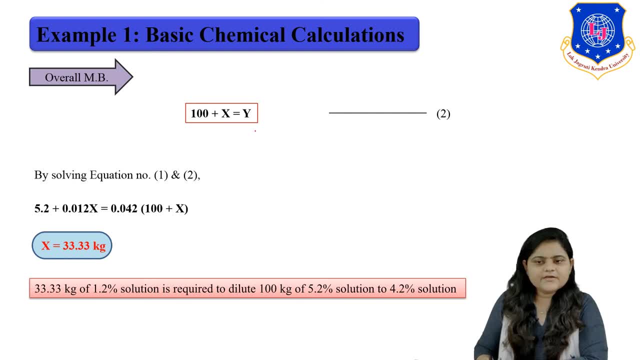 substituting the value of y, right. so value of y is nothing but the 100 plus x. so in the equation number 1 we are putting the value. of equation number 2. if you will solve this you will get answer is: x is equal to 33.33 kilogram. that means 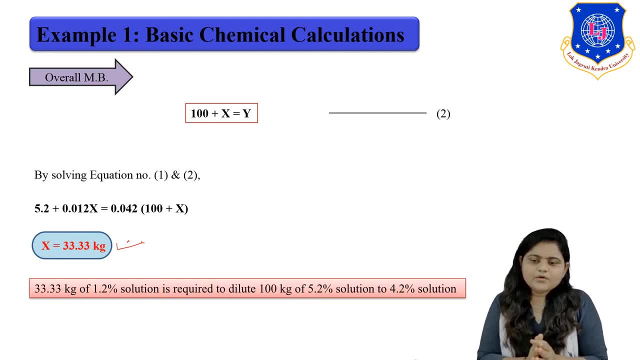 33.33 kilogram of 1.2 percent sugar solution is required to dilute 100 kilogram of 5.2 percent solution to make them 4.2 percent solution. so simply here i can say that in 100 kilogram of 5.2 percent sugar solution i need to add: 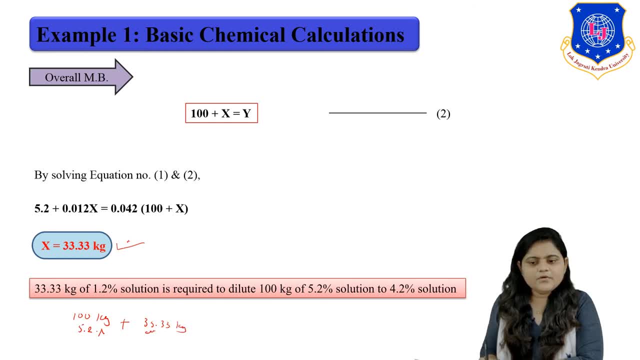 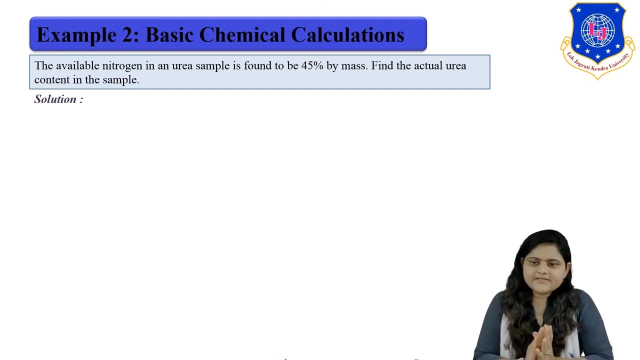 33.33 kilogram of 1.2 percent sugar solutions to make them 4.2 percent sugar solution. So this is a numerical based on the mass percent. Now let us solve one more numerical based on this mass percent concept. The given data is like this: The available nitrogen. 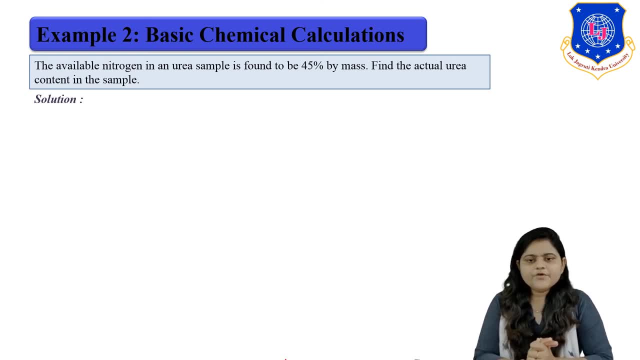 in an urea sample is found to be 45 percent by mass. Find the actual urea content in the sample. See meaning is very clear. Nitrogen in a known urea sample is found to be 45 percent by mass. Now we need to find out the actual. 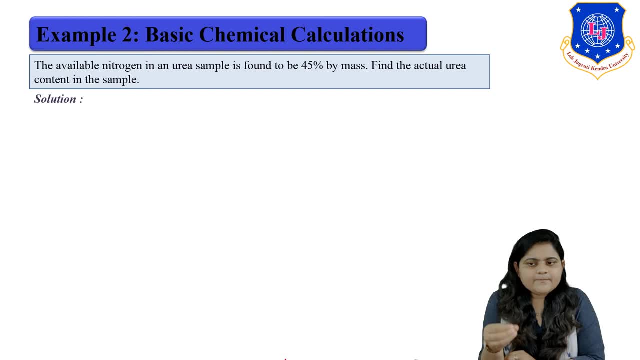 urea content in the sample. So whatever the sample you are taking, in which, what is the actual content of urea? here we need to find out the actual content of urea based on the nitrogen. Now in a some xyz sample, a nitrogen is found as 45 percent by mass. So first here, we need to assume a base. So let us assume a 100 kilogram urea as a base. But means: here we are assuming urea sample as 100 kilogram, Here we are assuming urea sample as 100 kilogram. In that 100 kilogram of urea sample, 45 percent by mass is the nitrogen. So amount of 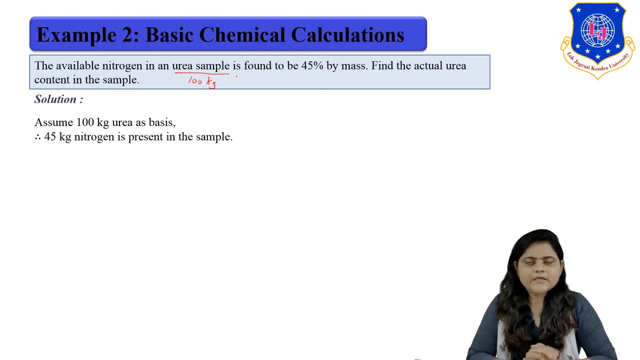 nitrogen in that sample will be 45 kilogram. Amount of nitrogen in given sample is 45 kilogram. So nasıl's question is here What? There is no where, and it can be explained by the number of wentocons. 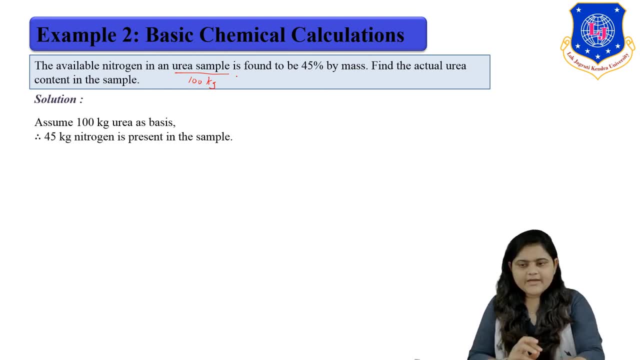 There is no where, and it can be explained by the number of went�� выбor. non 這個 수 그다음에 is 45 kilogram right Now. what is the molecular weight of urea? Right formula is NH2,, CO, NH2,. 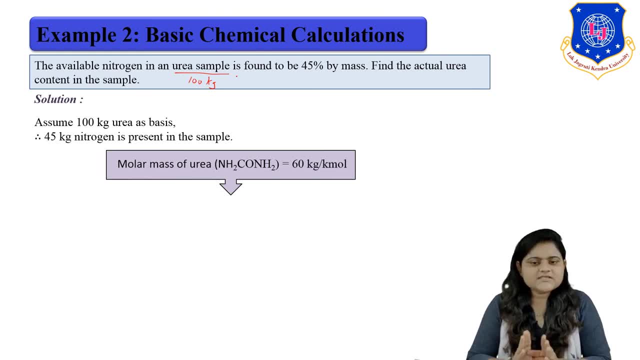 nitrogen 14, hydrogen 1, carbon 12, oxygen 16.. So molecular weight of urea will become 60 kilogram per kilomole. See in 60 kilogram per kilomole how many kilogram of nitrogen is. 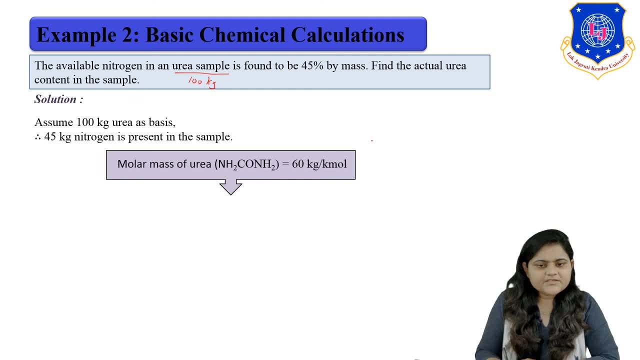 present. See how this 60 will become This: 14 plus 2 plus 12 plus 16 plus 14 plus 2, right? So by this way it will become 60. So in 60 kilogram of urea here I can say 14 plus 14,. 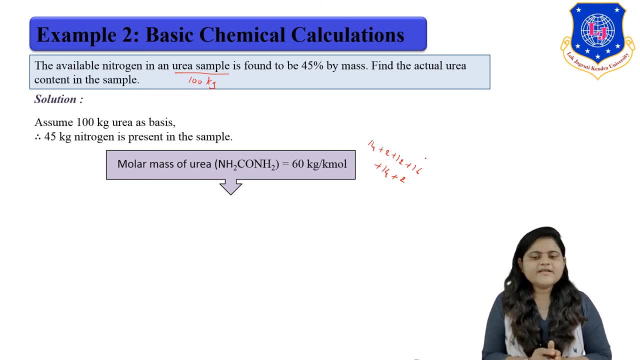 that means 28 kilogram of nitrogen is present. In 60 kilogram urea 28 kilogram nitrogen is present. So by this way it will become 60. So in 60 kilogram of urea here I can say 14 plus 14,. 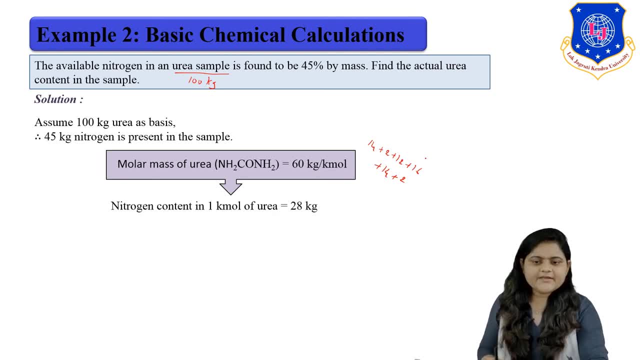 present, So nitrogen contained in 1 kilo mole of urea. 1 kilo mole of urea that means 60 kg. per kilo mole urea, nitrogen is 28 kilogram. So here I can put this equation like this: 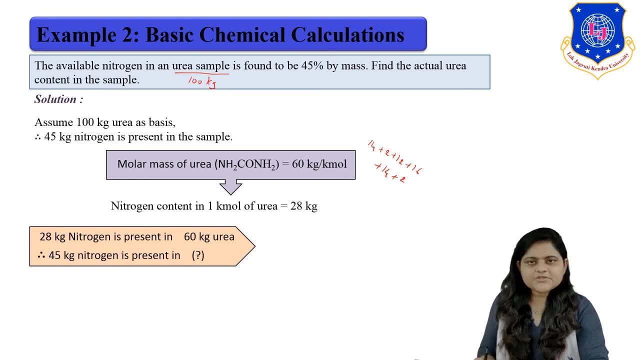 a 28 kilogram nitrogen is present. in how much quantity? 28 kilogram nitrogen is present in 60 kilogram urea. So if nitrogen present is 45 kilogram, so what will be the amount of urea? Again, I am repeating: 1 kilo mole of urea contains 28 kilogram of nitrogen. How this 28 kilograms? 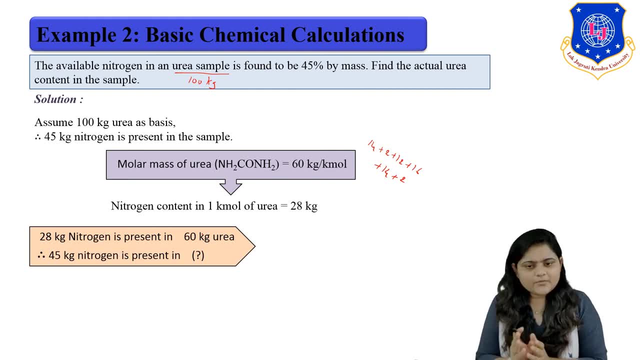 come Because the 60 kg per kilo mole, which is nothing but the molar mass of urea in that, 14 plus 14, that is 28.. So 60 kg. So 60 kg per kilo mole urea having 28 kilogram of nitrogen. Here we need to find out that if 45 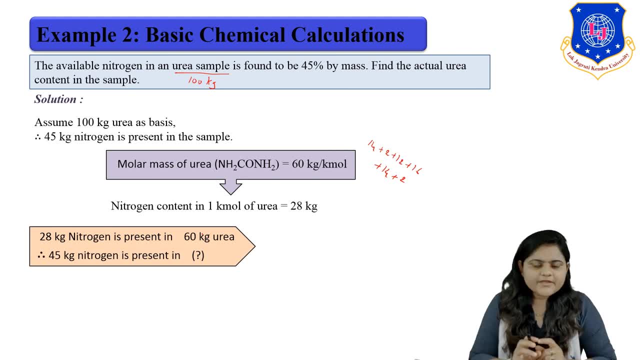 kg nitrogen is present, then what will be the amount of urea? So a 28 kilogram of urea is present in 60 kilogram urea. So if 45 kilogram nitrogen is there, then what will be the?